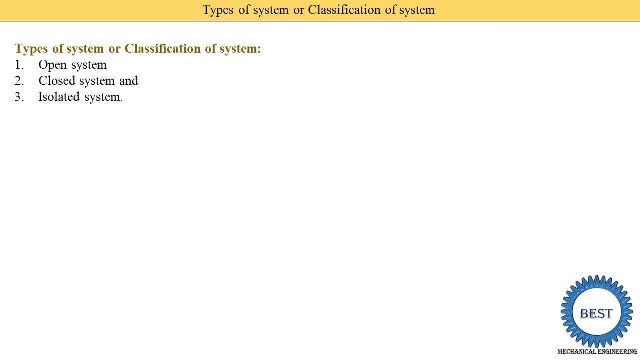 systems. I make the one separate video. So first we understand what is the closed system. So this classification is, or these types is given on the basis of mass transfer and on the basis of energy transfer. So on the basis of these two criteria, either the mass is transfer or energy is transfer. 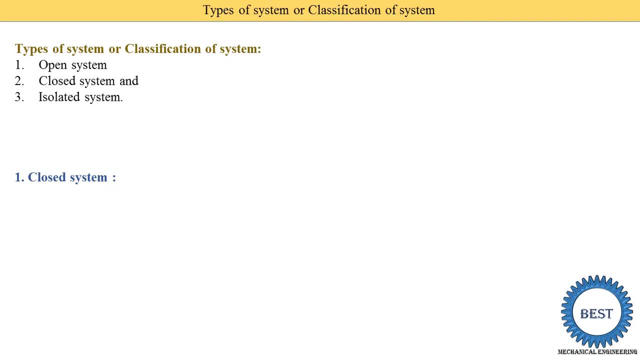 Energy means either the heat energy or work energy transfer. According to that the systems are classified. So from the name it is the closed system. Closed means there is a no mass transfer is there. That is a simple thing. So if anything is closed, then the no mass. 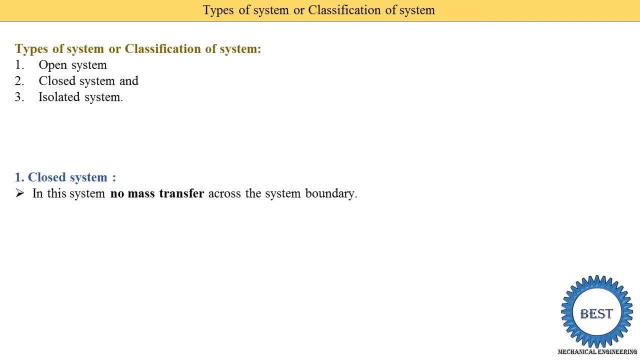 is able to enter inside. So this is called as the closed system. But in a closed system energy transfer is there. So in a closed system, from the name we understand, there is a no mass transfer. So in this system, no mass transfer across the system. boundary means. 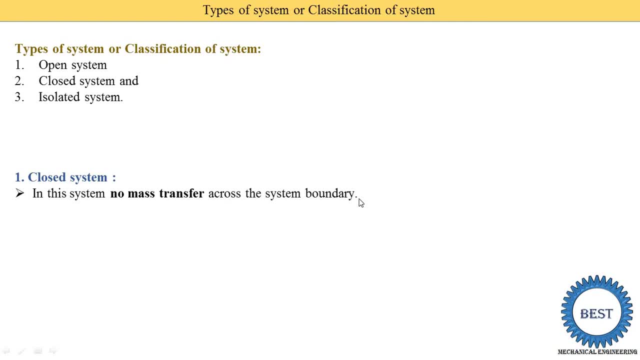 mass never enter into the system and they are not going out to the system or they are not cross the boundary. But energy in a form of heat or work can cross the boundary, as shown in this figure. So this is the image of the one cylinder and the piston. So this is the closed system. 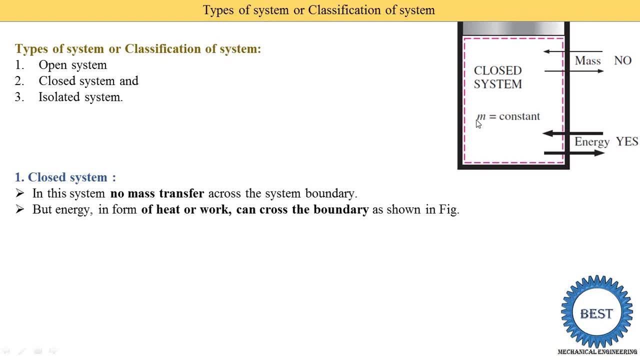 Here you see, that is the M is constant return. So that is, the M mass is already present inside the system and this mass is remains constant. So there is a no change in the mass transfer. So here you see, we return. that is a no means that is in and out of the mass here return. 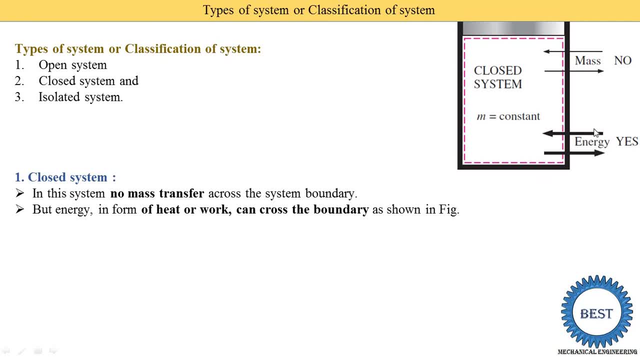 no means. that is a no mass transfer is there And here the energy interaction is there. Here the energy in, energy out And here return is the yes, Okay Means energy transfer is there? Energy means it is either the heat energy or the work energy can cross the boundary as shown in the figure. 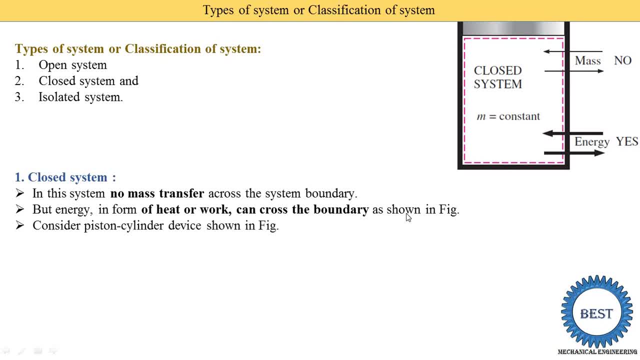 Now consider the piston cylinder device as shown in this figure. Okay, So this is the already piston cylinders. Okay, Then next what we do, the piston is move upper. this piston is moving in upper directions. Okay. When piston is moving in upper directions, When? 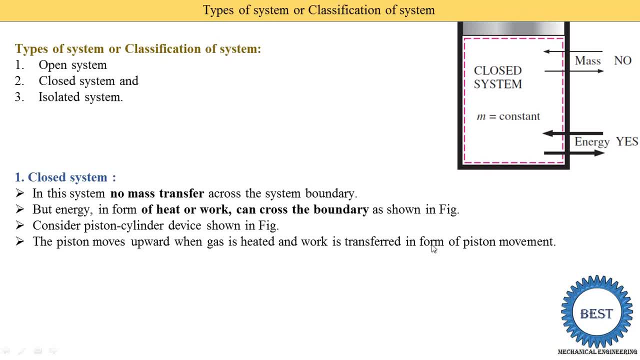 we hit this gas, Okay, And the work is transmitted in the form of piston moment. Now, here you see: we hit this gas, Okay. So due to the heating, the volume of the gas is start to expand. Okay, That is, a mass is already remains constant, But due to that, the pressure is increased. 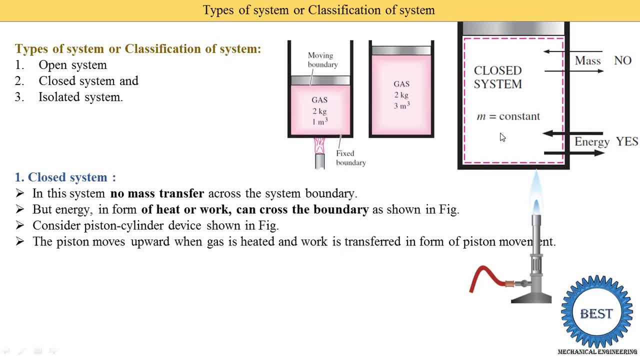 and due to the pressures, the piston is start to move. Okay, And it's give the little bit work done that is called as the work energy. Okay, Here we transfer the heat energy. Okay, And here the gas is 2 kg, volume is 1 meter cubes. 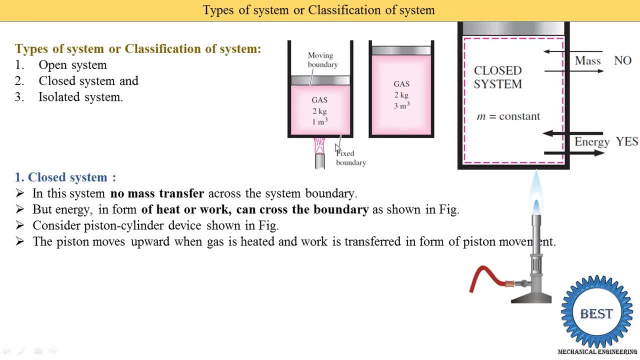 And this is the piston, and it is the moving piston. Okay, So when we give heat energy here, the volume is expand and due to this expansion of volume, this piston give some work done. Okay, So we supply the heat and what we get, we get the work done. That's why. 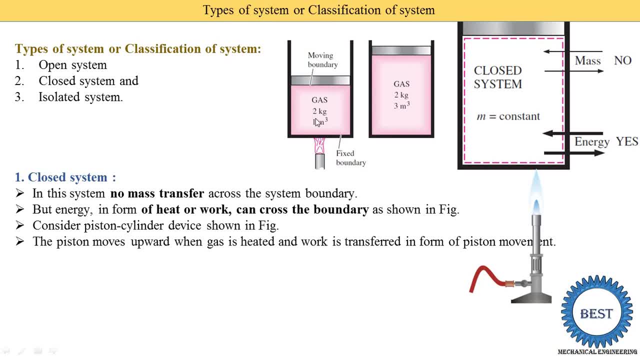 it is called as the flow system, But amount of the mass is remains constant. that is a 2 kg Here. you see, that is a mass, is 2 kg Means No new gas is added and not gas is going outside to the system. that is written in the first. 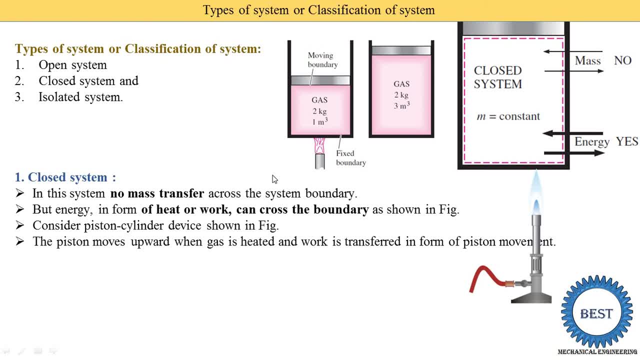 sentence: Okay, There is a no mass transfer across the system boundary. So already written that, but there is a no mass transfer across the boundary. Now we discuss the one examples, that is, a cylinder bounded by the piston with certain quantity of the fluids that we already 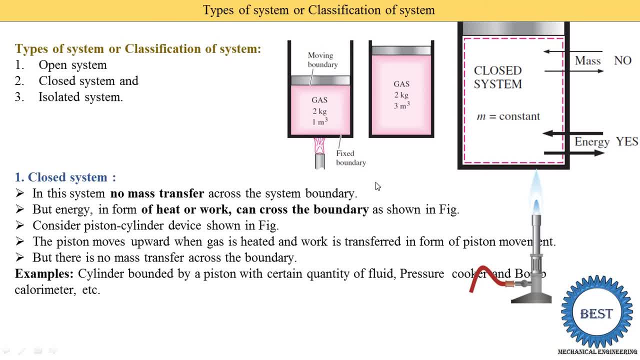 discuss here. Okay, That is a cylinder bounded by the pistons. Next one is the pressure Pressure cooker, and the bomb colorimiters are the examples of the close system. More examples I discuss at the end of the video with clear view. Okay, So pressure cooker. 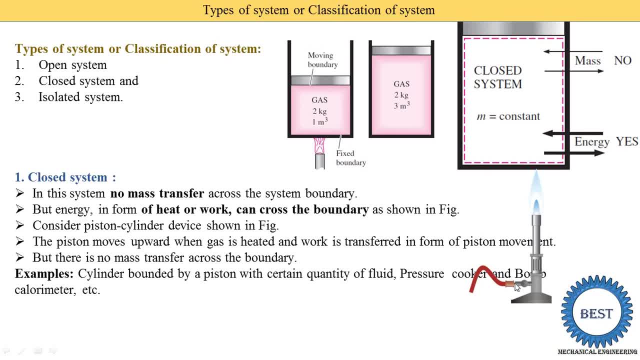 is considered a close system is the visual is not provide on that, Okay. So we have: when the visual is there, some quantity of the steam is coming out, Okay. When the pressure is too much increase and the bomb colorimeter is done. another examples of the close system. 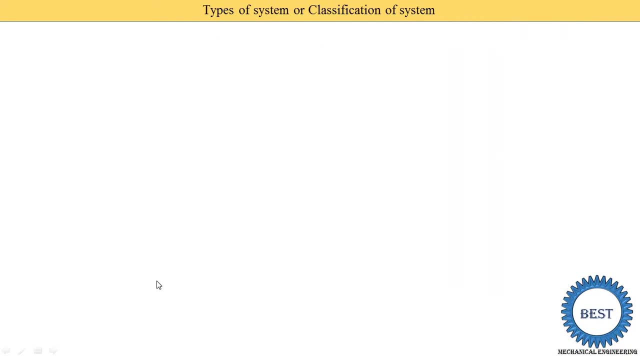 So in examination, there is a possibility of asking to select the MCQ: What is the open system? So in an examination, there is a possibility of asking to select the MCQ- What is the open system from the following option. so you need to select the correct system now before moving on the next. 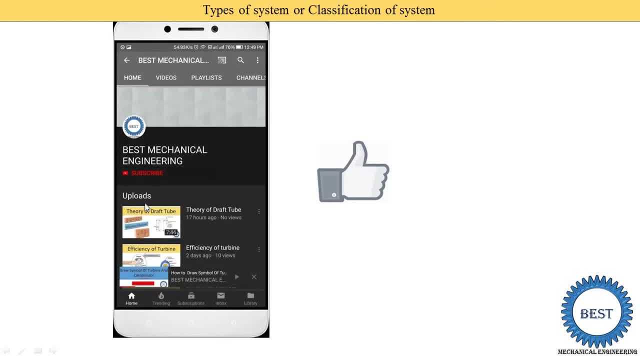 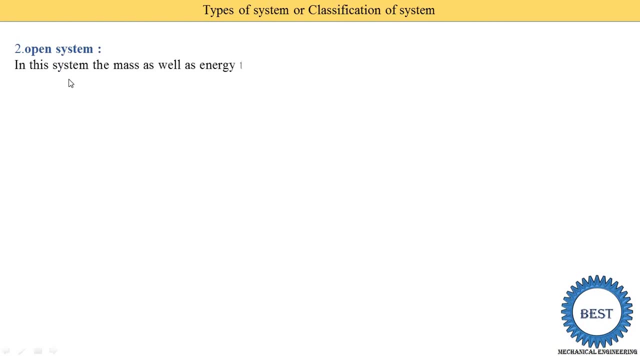 systems. i request to like the video and subscribe my channels for watching the more video related to the engineering, thermodynamics, as well as from the mechanical engineerings. for more video, i request to visit the playlist now. the next system is the open system. open means mass transfer is. 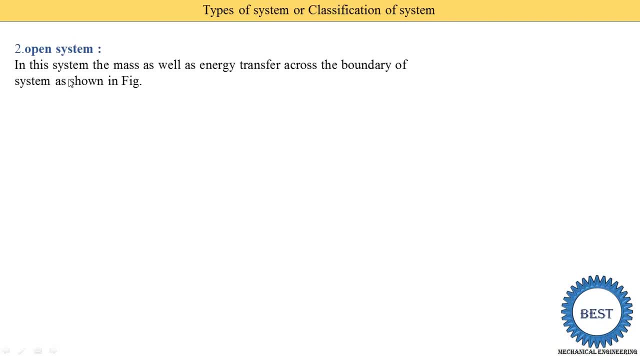 also takes place. energy transfer is also takes place. it is called as the open system. okay, so in this system, the mass as well as energy transfer across the boundary of the system, as in this figure, means mass interaction is also there, energy interaction is also there, and most. 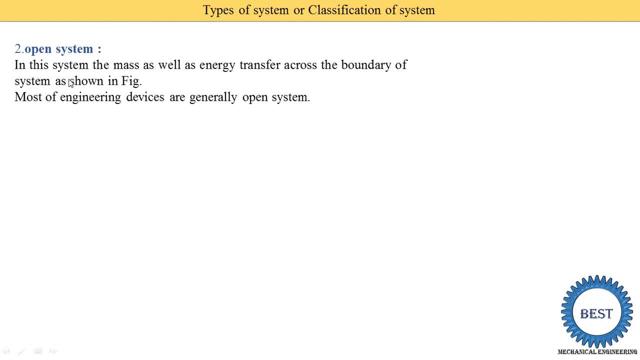 of the engineering device are generally open system. so majorities of the mechanical engineering systems are the open, open system. okay, now example is that in air compressors, gas turbine, steam turbine, refrigerators, and these are the examples of the open system and you also need to draw this figure in examinations. 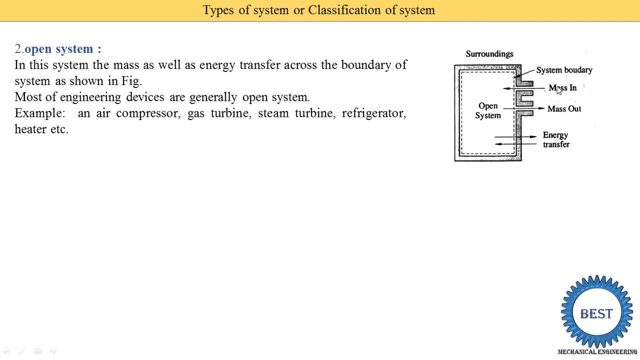 this is the open system here. you see, that is, a two opening is provided. okay, from one opening, mass is enter inside the system. from the second pot the mass is going out. okay, and this dotted line is the system boundary and energy transfer. we draw the energy transfer. 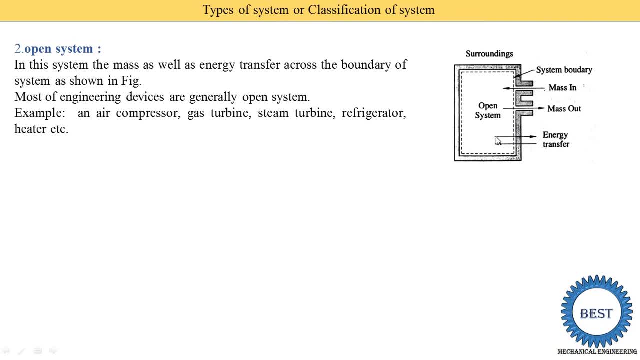 anywhere in this system. okay, so energy interaction is takes place in the form of heat as well as the work energy. okay, now in a air compressor. so air compressor is generally used to compress the air. okay, so we feel the compressed air in our tyre of the our vehicles. okay for that. 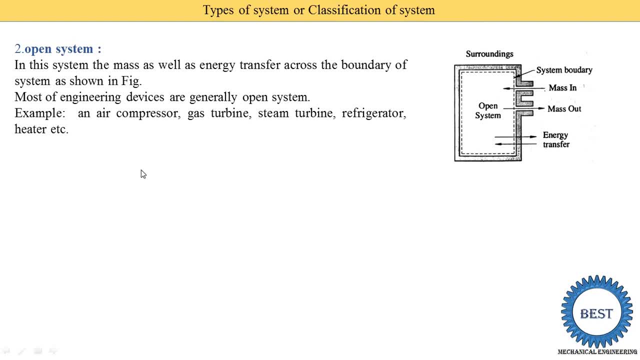 they require the compressors. okay, in a compressor we need to supply some work. okay, so some work is supplied to the compressor, that is, a mechanical work is supplied and due to compression, the pressure of the air is increase. with the pressure it's temperature is also increase and continue. 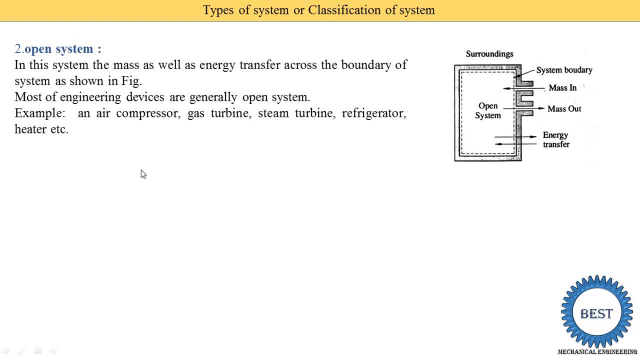 use new mass of the air is supply- okay, that's why it is called open system. and similarly, in a gas turbine, steam turbines, refrigerators and heaters are the open. various open systems. okay now. next one is the isolated system. more example of open system i discuss at the end of the video. next, 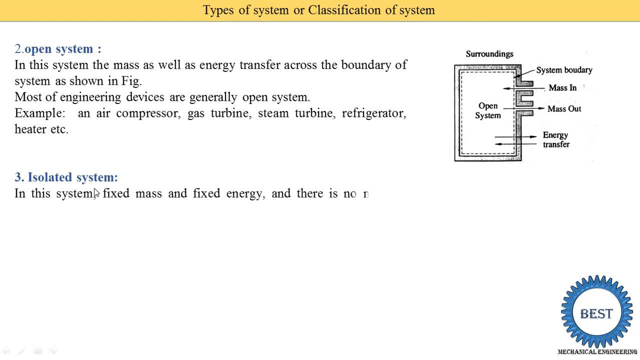 one is the isolated system. in this system, fixed mass and fixed energy means there is a no mass or energy transfer across the system. boundary, as shown in this figure, means in a such a system there is a no mass transfer is there and no energy transfer is there. that is called as 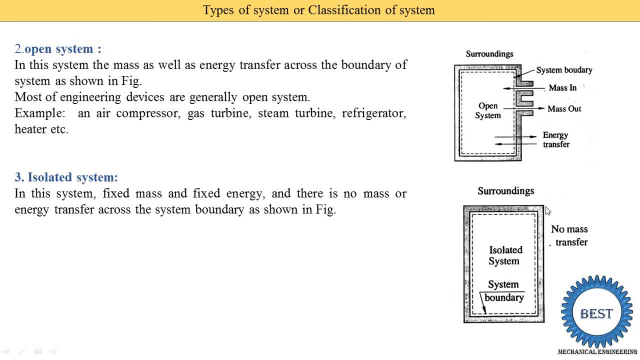 the isolated system. okay, so in this figure, you see, we draw one rectangle, this is the boundary, this dotted line, and here we return: isolated system. and this out outside part is the surrounding means. there is a no mass transfer and there is a no energy transfer is there, it is called as the isolated 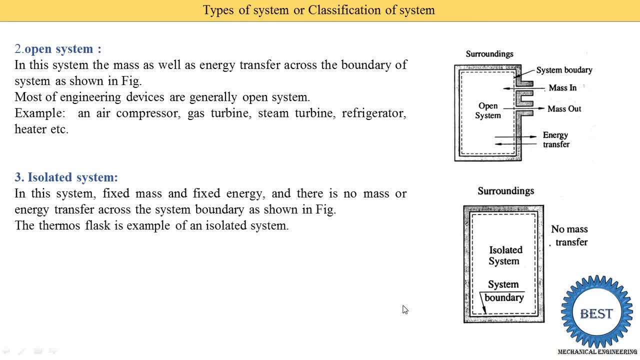 system. okay, the thermos flex is examples of an isolated system. generally, we you use the thermos flag for the, the store, the t and that. okay, to maintain the temperature of the tea water. okay, that is called as the thermos place, but actually there is a. no system in this world are the. 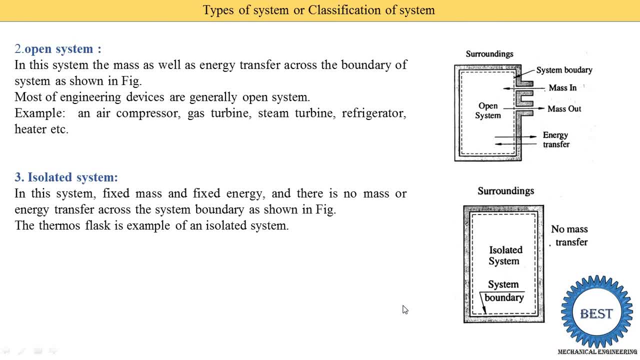 isolated systems. because in thermos, thermos place even the t is also cooled down, or any food is the cool down after the some times? okay, so in this world there is a no system. is the isolated system? now here i discuss the few of the examples. okay, 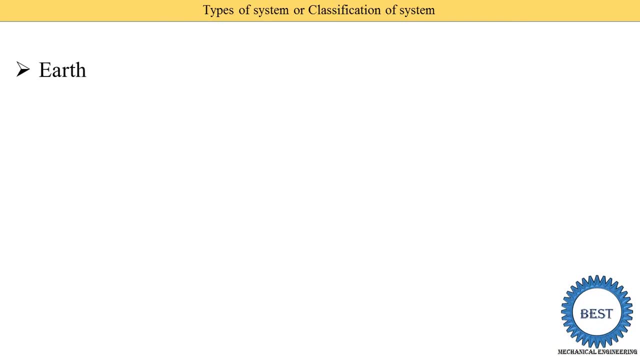 now, art is open system, close system or isolated system. okay, so art is the open system because the our atmosphere is the our boundary for the art. okay, so there is a no mass transfer is there from this layer of the atmosphere. okay, in some case, there is a mass transfer, is that? 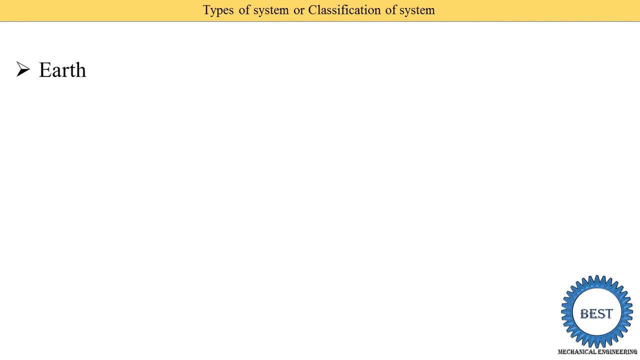 satellite is going inside and outside. so that is a minor thing, is there? okay, but there is a energy transfer. is that solar radiation is coming on, that some of the solar radiation is again reflected to the back, to the atmosphere? okay, so this art is called as the 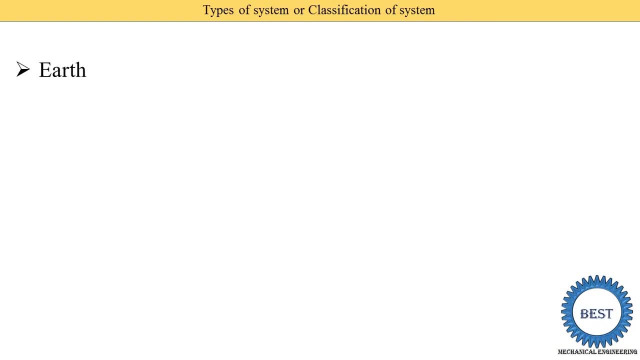 closed system, not an open system. it is the closed system, that is, a energy interaction is there, but there is no mass transfer, so it is called as the closed system. second one is the human body. so in human body is the open system. why it is open system? because we inhale the oxygens. 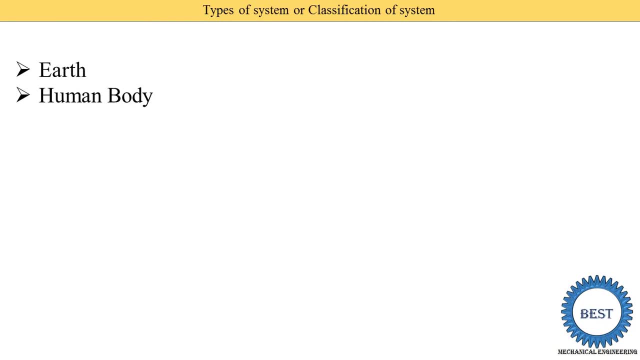 we drink the water, we eat the food. we remove the co2- okay, and some another waste in the morning. so our body is the open system, because our body is also transferred the heat energy, because we feel the hot and cold in a different seasons, so our body also do the heat interactions. we are performing some work, so energy and heat transfer. 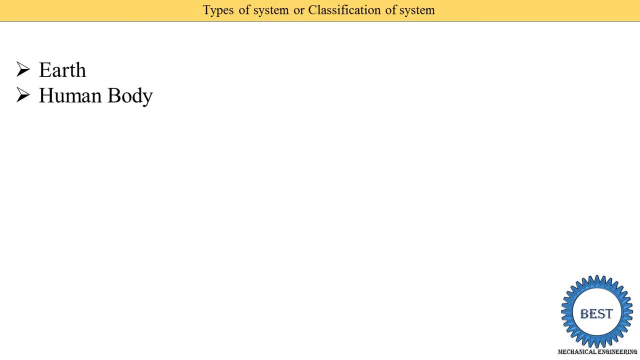 both are there and we also transfer the mass because we continuously take the oxygen. okay, we drink water, we eat the foods. that's why the human body is the open system. now, here there is a two confusing thing is there. one is the refrigerators and second one is the. 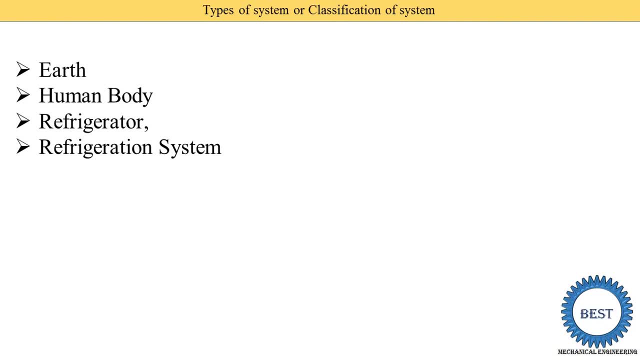 refrigeration system. refrigerator means the freeze available at our home that we use for the storage of milk, storage of waters, storage of fruits- okay- and storage of the vegetables. so in the refrigerators we putting the different foods, okay, its temperature is reduced, means energy transfer is there. 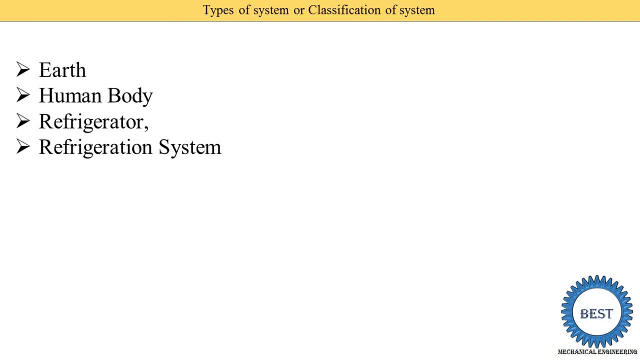 for the cooling, we supplied the electricity to the refrigerators. okay, and we also changing the mass. we remove the milk, we put the milk, we remove the vegetables, we put the vegetables. so it is the open system okay, but when we the, we think about the refrigerator. we put the vegetables, we put the. 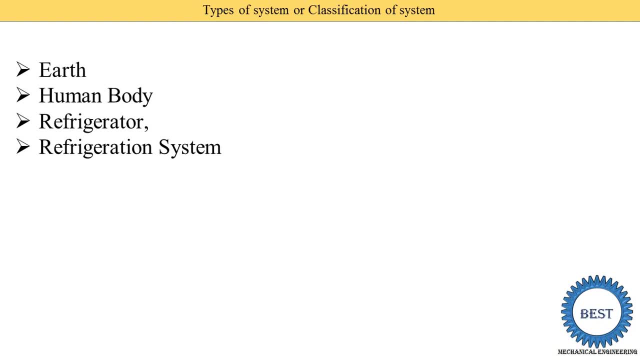 thinking the questions like the refrigeration system. refrigeration system means the compressor, condenser, expansion device and evaporator. okay, so these systems, refrigeration system- is considered as the closed system, but refrigerator devices come. then we say that it is the open system. okay, because in refrigeration system, in a four component, the one, refrigerant, means 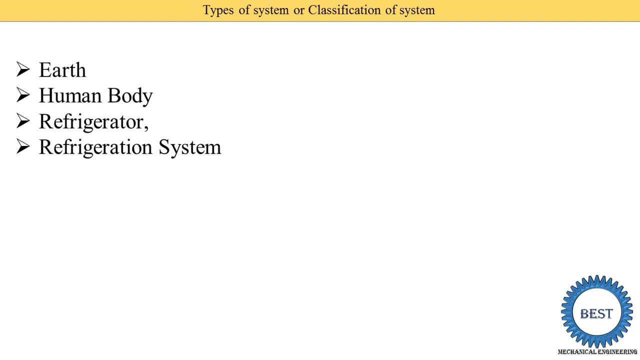 gas is circulated, so mass of this refrigerant is constant. okay, and we transfer the work to this refrigerant and we remove the heat and we supplied the heat in this refrigerant. that's why it is called, as the refrigeration system is considered as the closed system. 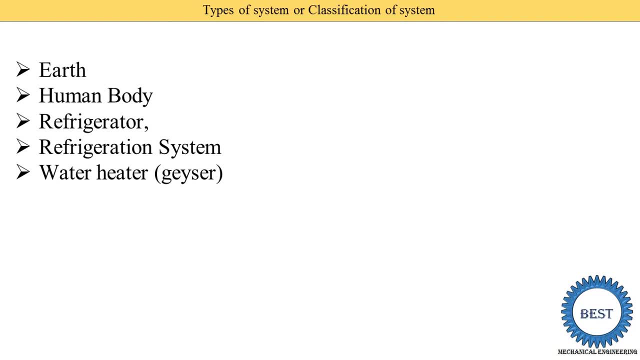 now. next one is the water heater. that is generally we used to for our bad purpose. okay, we create the hot water in a water heater or a geysers for our bathing purpose? okay, so what? the water heater is considered open, closed or isolated systems, so i don't explain about the water.